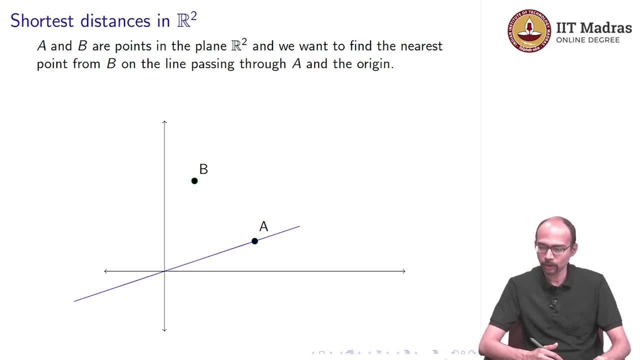 plane R2, you have two points, A and B, and you draw the line joining A with D, So that is the blue line in the picture, And now we want to find the nearest point from B on the line passing through A and the origin. This is what we want to do, So this 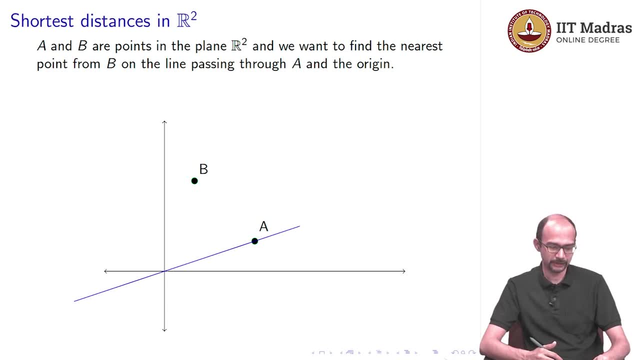 is maybe something that you have done in high school, meaning in your- I am not even sure- seventh or eighth standard, where we do geometry, we actually do this using the ruler and compass the compass. place it on B, then you draw an arc. it intersects the line in two places. 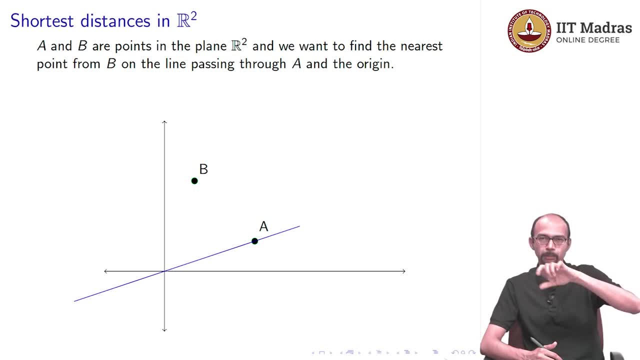 and you take your arc again, you draw- sorry, your compass- again, draw two arcs and then you join this and that sort of that is a perpendicular passing through this line And that perpendicular is actually the shortest distance of B from this line. So this is: 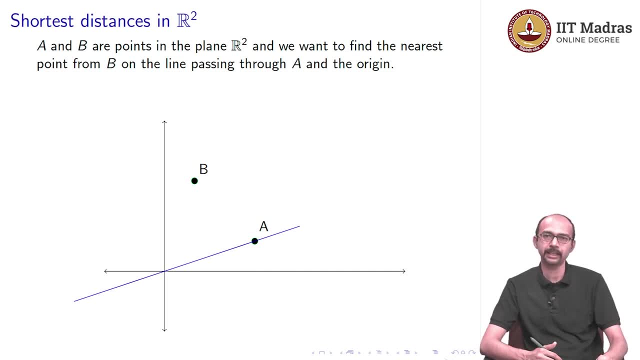 the shortest distance of B from this line. So this is the shortest distance of B from this line. This is what these are ideas that we have seen in high school geometry. So now I want to do the same thing using a little bit more sophisticated machinery. We do not actually. 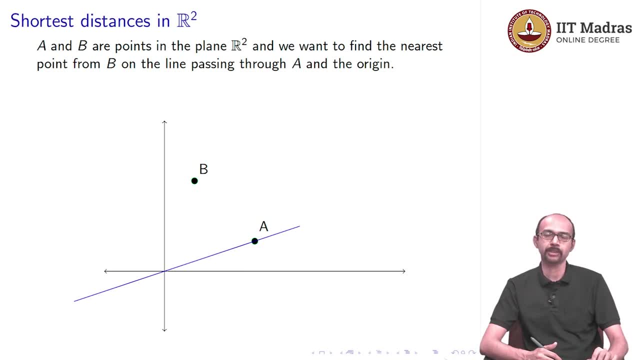 want to draw this. We are not interested in drawing it per se. What we want to do is to determine it. Is there a way of writing down equations in order to get the shortest distance? Is there a way to write down equations to get the nearest point? 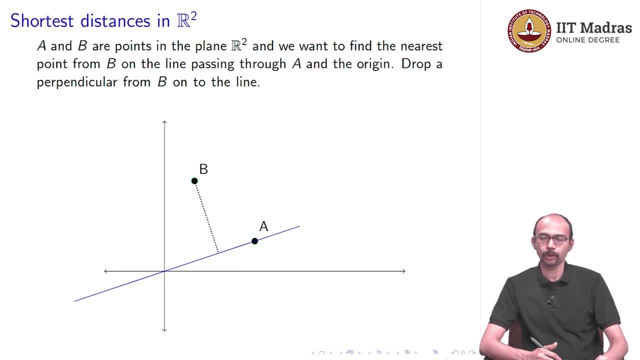 So drop a perpendicular from B onto the line. You can use the procedure that I just mentioned in order to do that. So the procedure that we have, using the compass and so on, that will tell you what the point is meaning. geometrically, you can identify what the point. 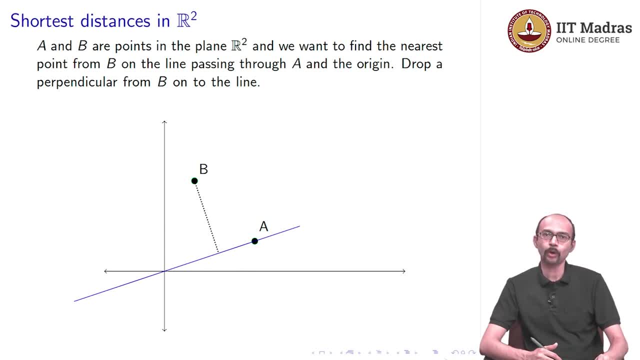 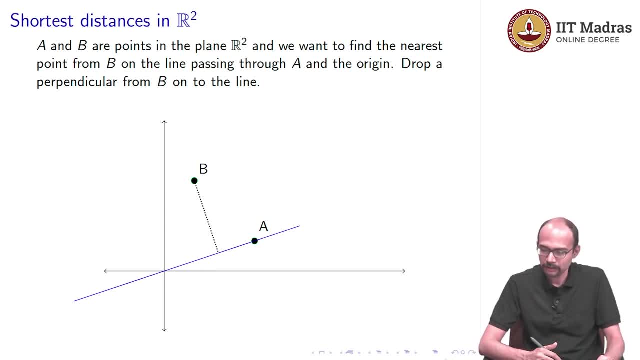 let us see how to do that. So now we introduce vectors. So this is where vectors start coming. So draw the vectors corresponding to the points A and B. let us call these vectors little a and little b respectively. And now let us use these vectors in order to determine what is. 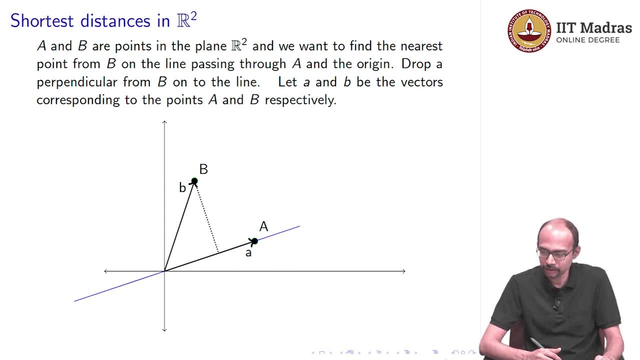 this point. So I want to determine what is this point. So let me that point. it is this point here, that is the point that we want. So let us see how to get that point. So suppose I know that this angle is theta, or I do not know the angle. 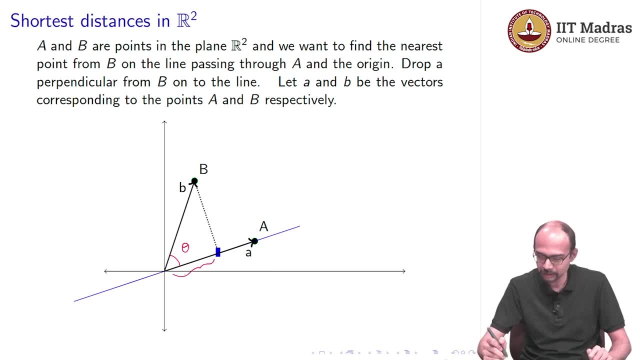 is theta, but I know the length of this line. If I know the length of this line, then I am done, because the point A is given to me. that is so. that means I can get the vector A. And then what I want to do is: I can, I want to scale this vector, because this is 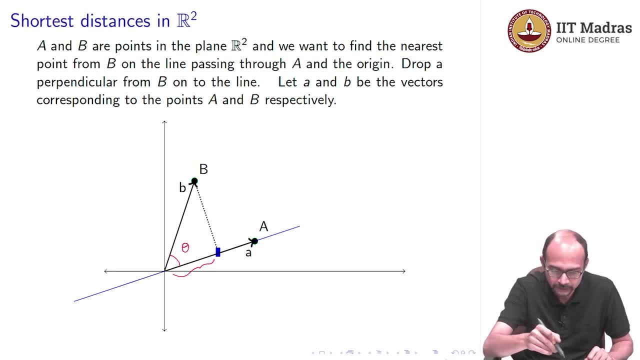 the vector corresponding to the point that I want. Let us do that in green. So the vector that corresponding to the point I want, that is this vector. here is some scaled version of A. So the vector I want, let us call it V. So V is equal to some alpha times A. This 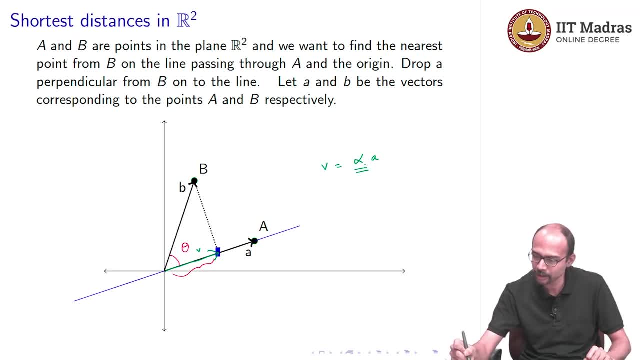 V is alpha times A, So all I need to do is to determine what is alpha, and then I can get what is. what is this point So? and what is alpha? Alpha is exactly going to be determined by this length in red that we have denoted here. So how do I get alpha? So what we 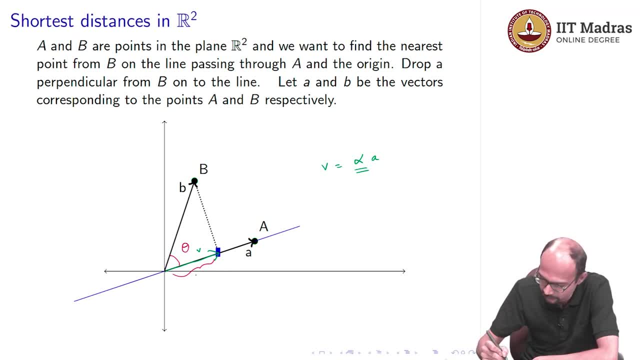 know, is. so suppose this length is given by, so this is essentially the norm of V, the distance of V from this point. So this is the norm of V. So the norm of V is what we want. So if we put it into this, 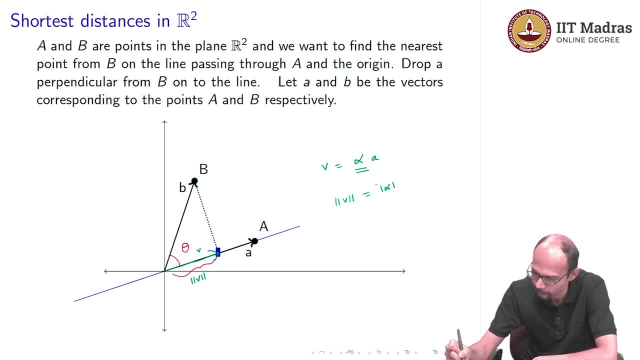 equation. this is mod of alpha, but we know that alpha is actually positive, So we do not need to put the mod alpha times norm of A, which means alpha is equal to norm of V divided by norm of A. So in other words, V is equal to norm of. 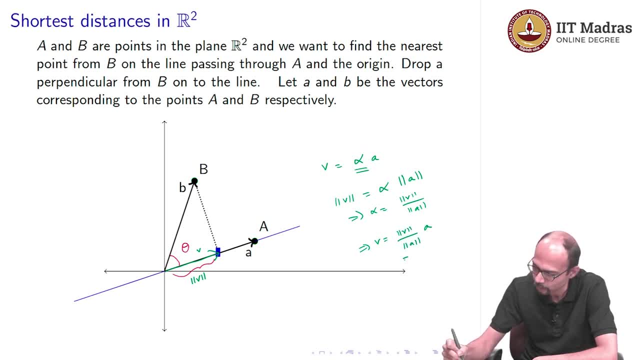 V divided by norm of A times A, or in other words, norm of V times A by norm of A. So you can see, A by norm of A is a unit vector, Meaning it is a vector of length, 1.. And then, 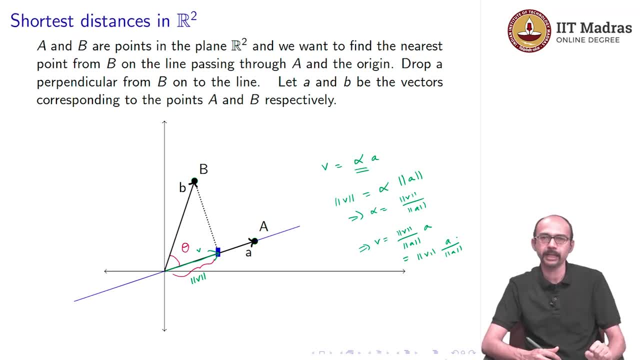 you, when you multiply in the same direction as A, and then when you multiply it by norm V, we will get exactly V. So now I know A, because I now the point capital A, and once I know a, I can determine what is the norm of A. So what I really need to know is what. 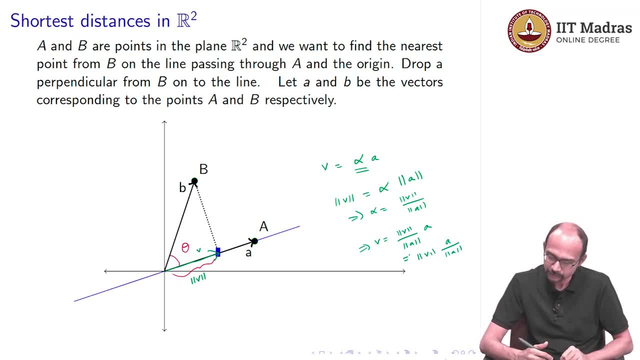 is norm of V And for norm of V, well, we know that norm of V is equal to the norm of the vector B times cosine theta. This is something we know from our Euclidean geometry, or this is the definition of cosine of an angle. It is the length of the adjacent side divided. 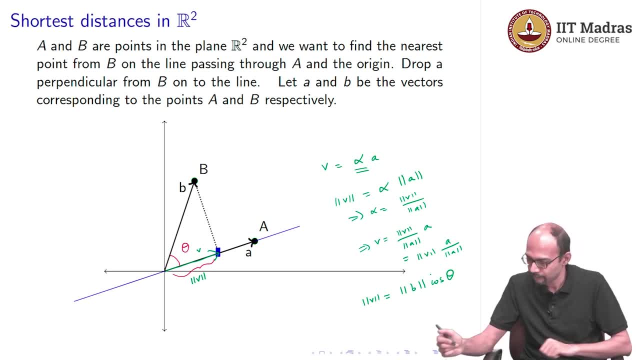 by the length of the hypotenuse. So I know this is norm of V times cosine of theta. but now I know what is cosine of theta. that is exactly where. so so far I have only used the lengths, but now I will use the inner product because the cosine of theta, remember. 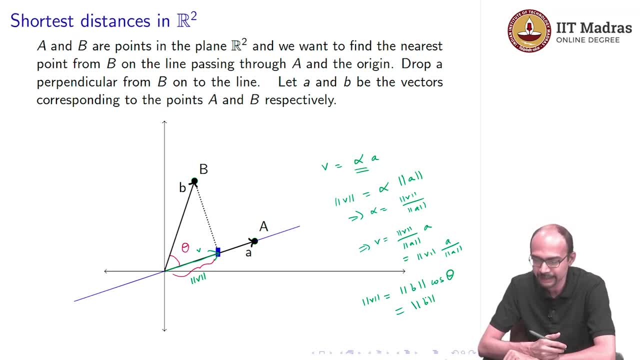 theta is also the angle. it is not just the angle between B and V, it is also the angle between B and A, And so I can write down cosine of theta as the inner product of the ívork of A comma B, I mean in terms of the inner product of A comma B. so this A. 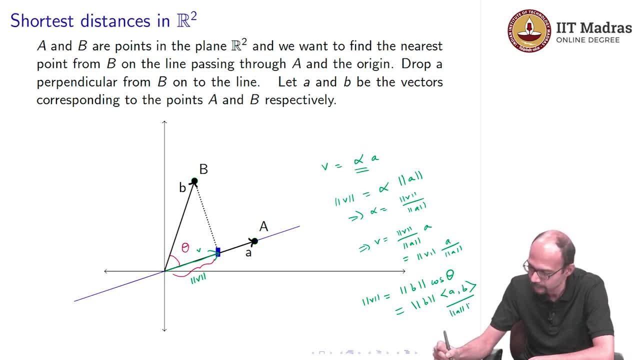 comma B divided by norm of A, norm of B. If I put all of that together, what we are going to get this: that V is equal to norm of V times A by norm A, which is equal to norm of B times inner product of A. Ourenc resize class, the value of A and the inclined axis. 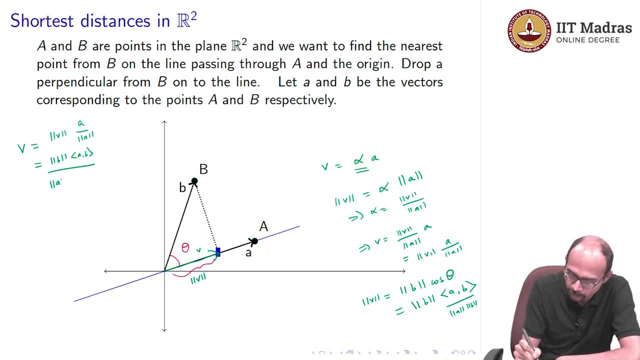 What 2 is, because this is, along to 0.7 никтоis, Cu 1 into 1, C1 into 1, by A root 6 multiplied by product of a comma, b by norm of a, norm of b, a times norm of a, and these two norm of b cancel. 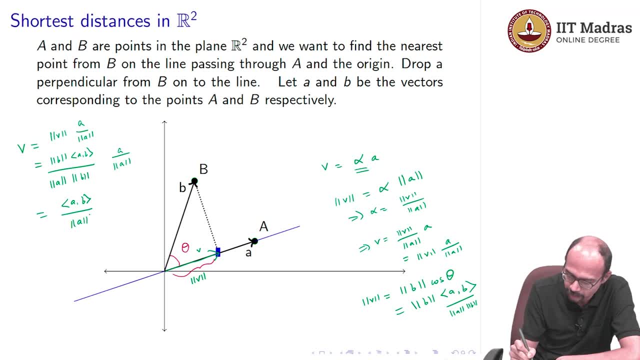 So this is inner product of a comma b by norm of a squared times a, and I can write this: since I have a norm of a squared, I can write this as a comma b, inner product of a comma b divided by inner product of a comma a times a. So that is what we get. So if you know a and b, 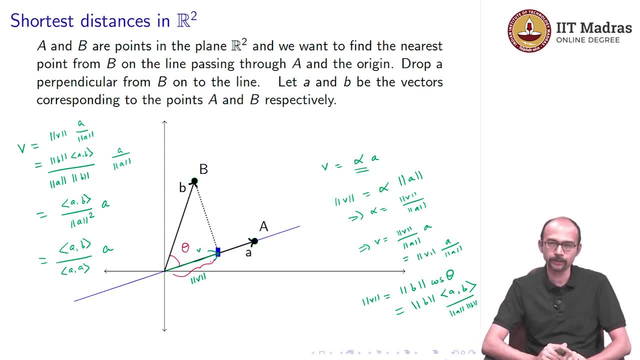 well, I know what is this? vector v, which is the vector corresponding to the point that I wanted. that was the nearest point on this line, So you can see how we have progressed from Euclidean geometry to coordinate geometry, to vector geometry, which helped us solve the 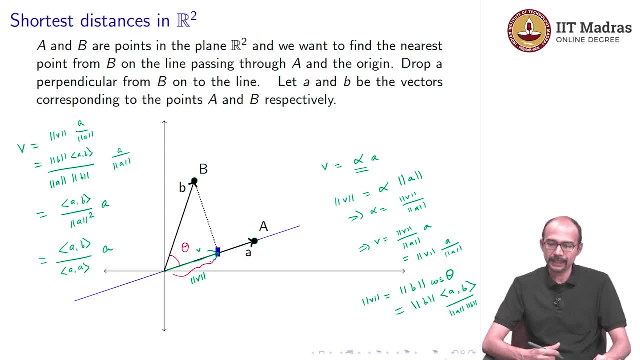 problem in coordinate geometry, And the point here is that we used the inner product very crucially to get what we wanted. So in this case, of course, the inner product is just the dot product. So when I said inner product here, I meant the dot product. So this is ab cosine theta. 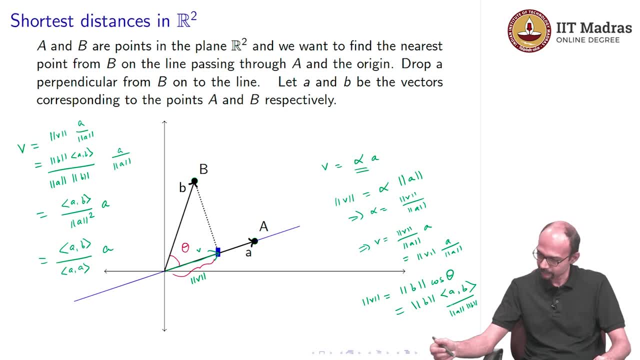 I mean, this is so. that is what I used here. So a dot b is equal to length of a times length of b times cosine theta. That is what I used here. So this is a rather expansive discussion about the nearest point. So let us also recall what the 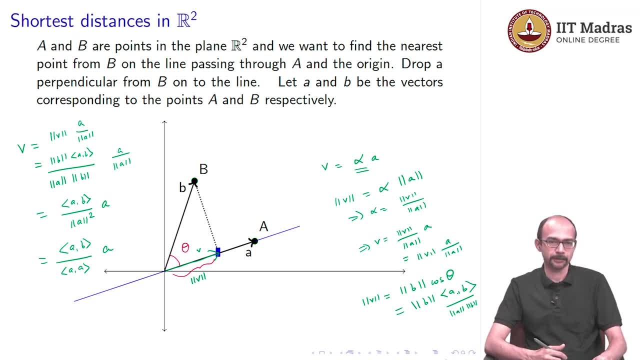 nearest point tells us in terms of shadows, because that is really what projections are. So suppose there is a light source over here which is emitting light. it is right on top of b, on top in the sense of this perpendicular, And if you have the light coming out like this, then 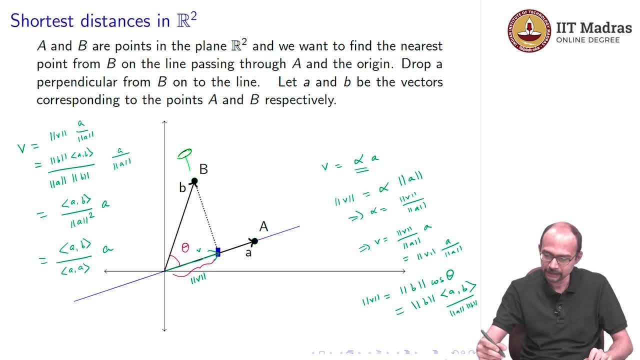 the shadow of this vector is going to fall exactly where the green line is on v. So this is what a projection does: It takes, it, takes something and projects it down to something else. It is as if there is a light source behind, And when we do a usual inner 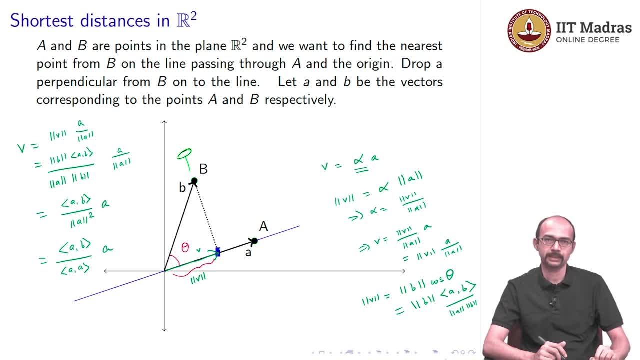 products and usual lengths and so on. then that means it is perpendicular. It is like the shadow is falling exactly perpendicular to what is below. But we will see things which are not like that also, and there we will actually have to use inner products. the dot product will be. 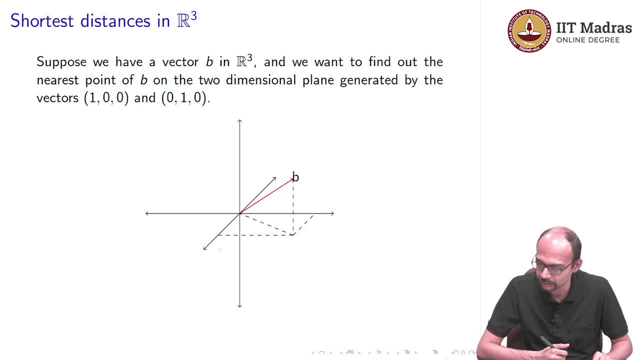 that is what this video is about. Let us quickly look at an example with the same idea. So here we have a vector b in R3, that is, the vector in red- And we want to find the nearest point to b. So this is not off. this should have been a 2,. 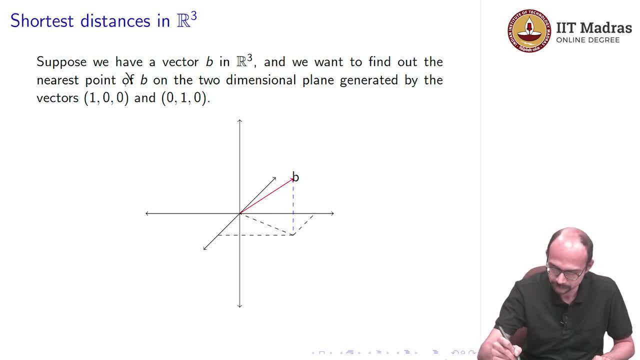 So the nearest point to be on the two-dimensional plane generated by the vectors 1, 0, 0 and 0, 1, 0, that is the xy plane. So what do you do? You drop a perpendicular. again the same idea, and then that point is exactly the point which. 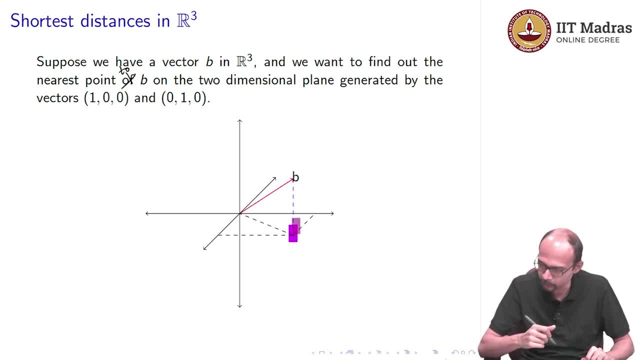 is closest. So this point here is the closest point. And how would I determine this point now? So, to determine this point again, you would go through the same ideas that we did before, So you would consider this angle, this angle is theta, and then you would work out the. 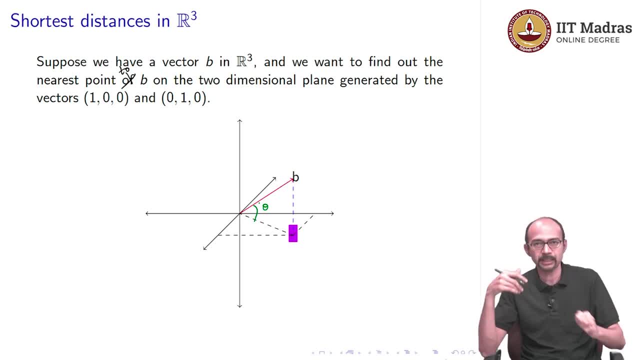 same. work it out in the same way, except here we do not have an, a, So instead of a we will have to use the vectors 1, 0, 0 and 0, 1, 0, and we will see. 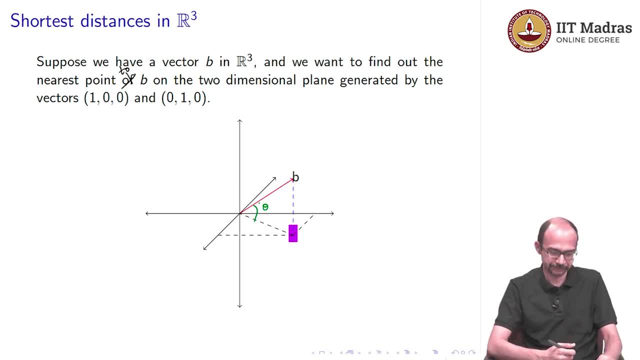 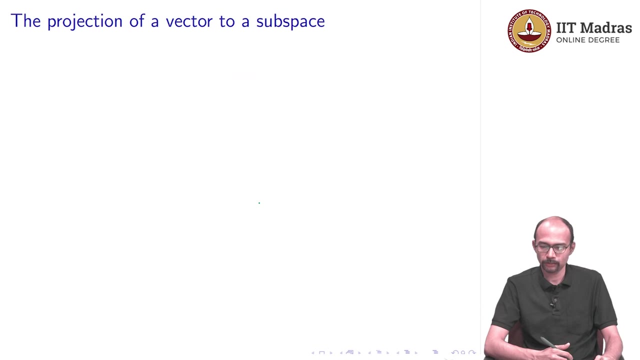 explicitly how to do that in a few minutes. The idea is going to be the same. We have to use the dot product and the lengths in a very effective way, So let us go ahead. What is the projection of a vector to a subspace? 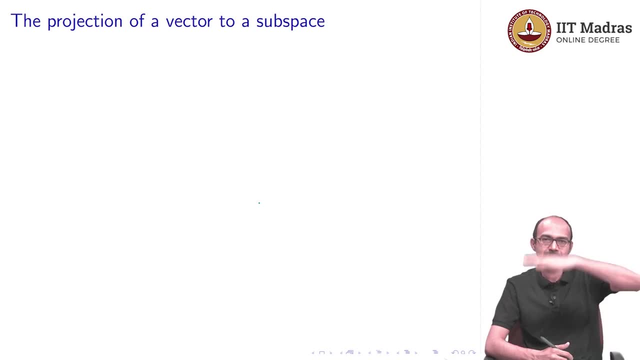 So we have seen two examples of taking this idea of shadows. Now let us do a general definition and we will see that the particular case of Rn, with the usual, with the dot product and so on, gives you the shadow that we just saw in the. 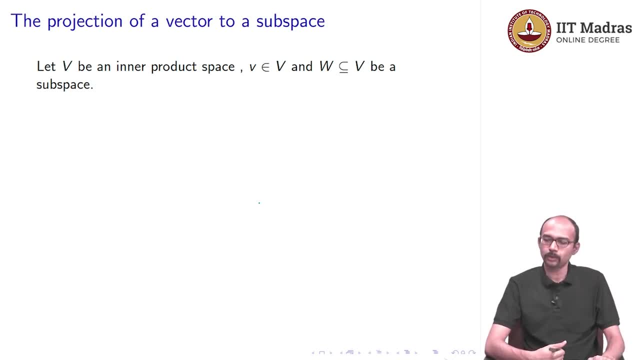 previous examples. So let V be an inner product space, you have a vector V, you have a subspace W, then the projection of V onto W is a vector in W, denoted by projection of V, subscript W, computed as follows- And I want to underline that I am saying computed and not defined: 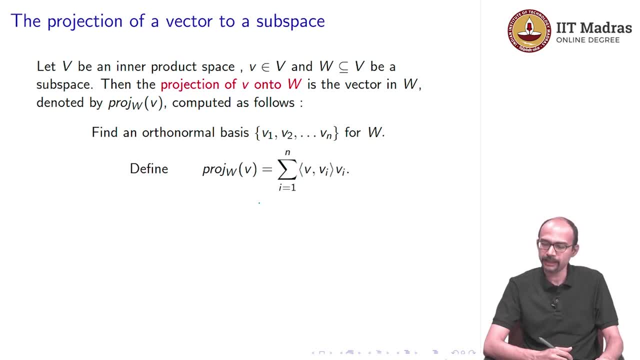 Find an orthonormal basis: V1, V2, Vn for W. Define the projection as summation: V comma, Vi times Vi. Okay, So now what happened here? Well, we took an orthonormal basis, which is why we did not have to divide by anything. 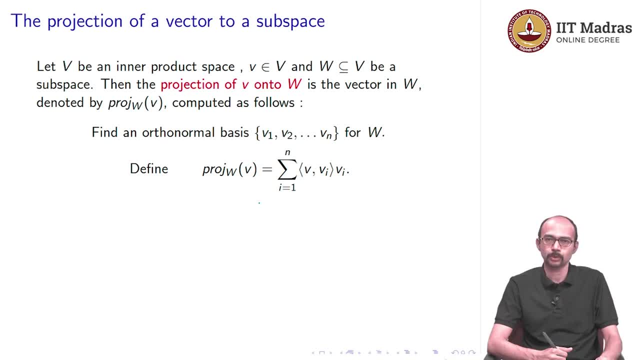 In our first example, remember, we had to divide by something, So the inner product of A with itself, so the norm of A squared. But since here our basis vectors are of length 1, we do not have to do that. 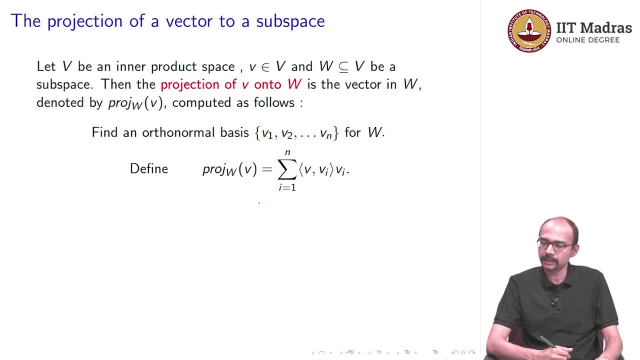 Here length means norm. So here you just take the inner product of V with Vi And multiply that number with Vi, and that is the projection of V onto W. You might identify this with something we saw in our previous video. So here is the main fact, which is why I said computed and not defined. 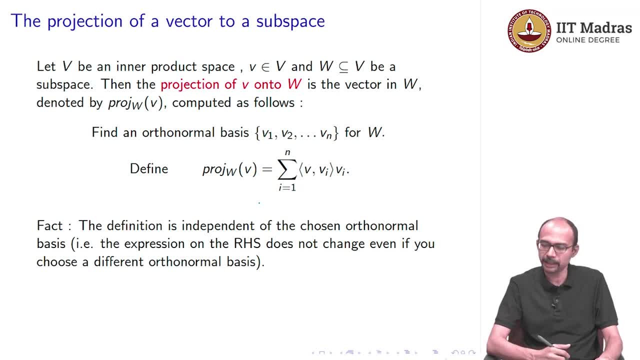 The definition is independent, or I should have said the expression is independent of the chosen orthonormal basis. What does that mean? The expression on the right hand side does not change. So when I say the expression, that means this expression here. 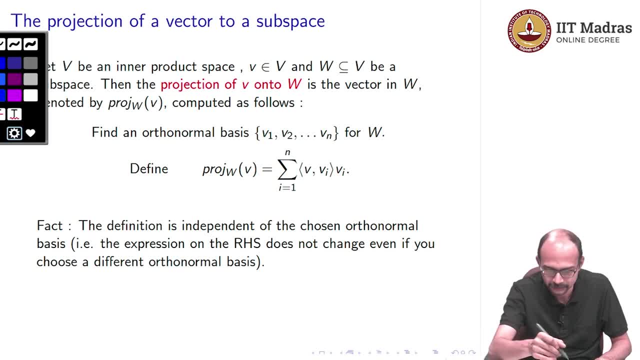 So the expression on the right hand side does not change. So when I say the expression, that means this expression here. This expression does not change, even if you choose a different orthonormal basis. So if I choose V1,, V2, Vn and you choose W1,, W2, Wn, then even then this will not. 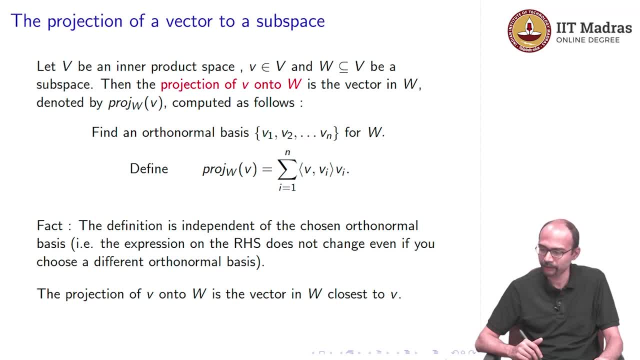 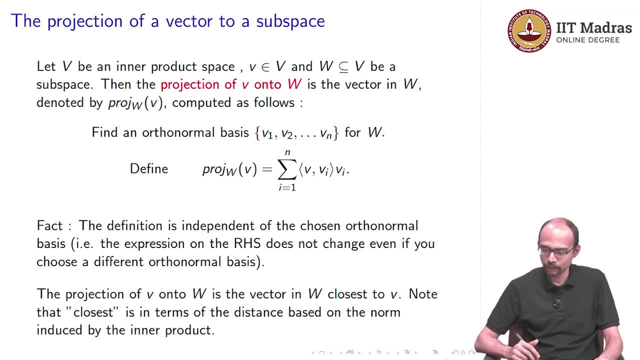 So the projection of V onto W is the vector and W closest to this. So the projection of V onto W is the vector and W closest to this. So the projection of V on this. So the projection of V on this. 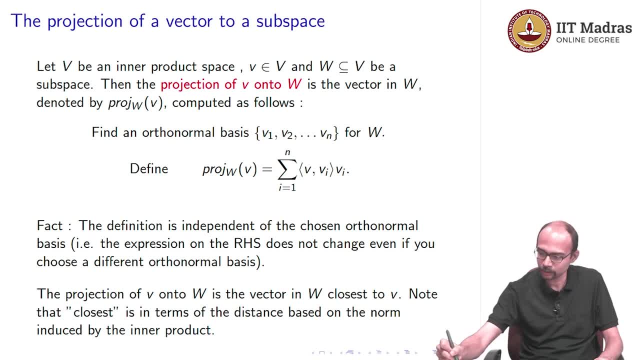 And what do we mean by closest? So note that closest is in terms of the distance based on the norm induced by the inner product. So what we mean is that if you take the smallest value of V minus W, so find W in. 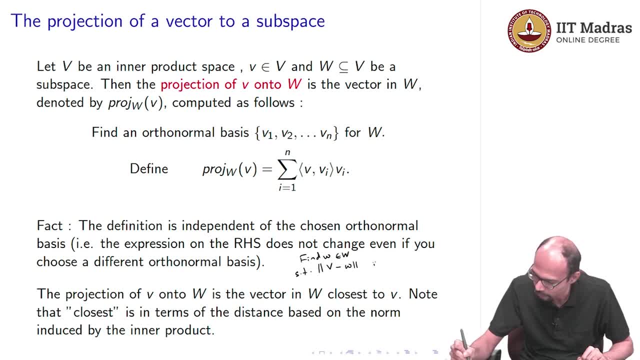 W such that this norm is independent. So what do we mean? norm is smallest. The answer is: w is equal to projection of v onto w. That is what we mean by the smallest distance. And here, what do we mean by distance? Because this is in the product space. there is no natural. 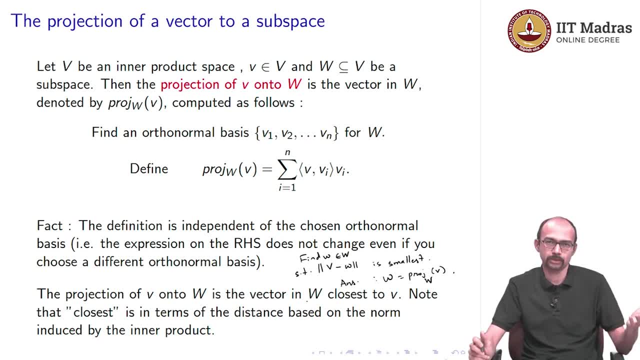 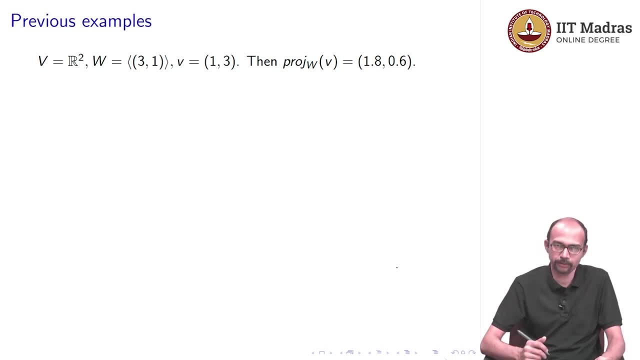 I mean there is no distance in the sense of length. that we have done for Rn. Here distance means the norm, Distance means norm. So in terms of the norm this is the smallest. Let us do examples. So I believe the previous definition may have been a little. 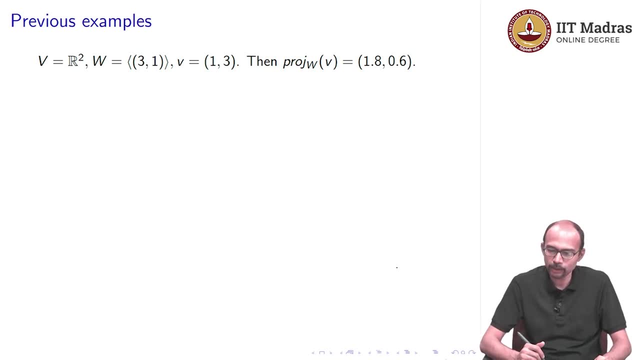 intimidating. So let us do some examples. So let v be R2 and let w be the subspace generated by 3 comma 1. And let v be 1 comma 3.. Then the projection of v onto w is 1.8 comma 0.6.. 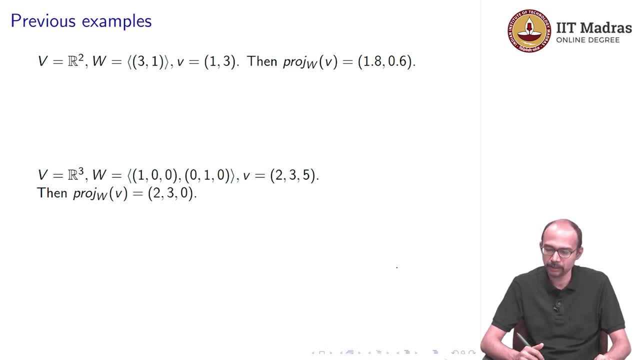 Similarly, if v is R3 and w is the subspace generated by 100 and 010, so that is the xy plane, and you take v to be 235, then the projection of v onto w is 230.. Let us work out these examples and it will make it clearer what we mean. First of all, 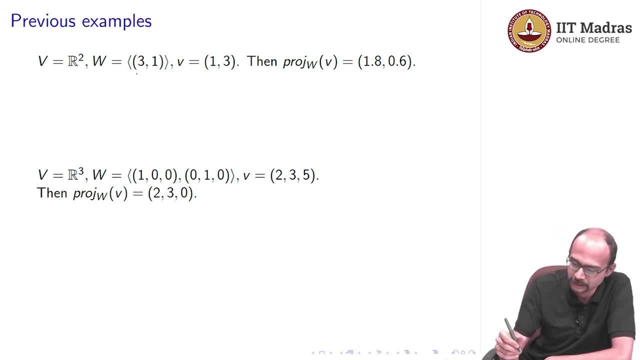 if I have an orthonormal basis for the vector space at w at hand. so here, if you take 3 comma 1 and divide it by root, 10, so this is an orthonormal basis for w. Now let us take v And then by definition you have to take V comma this. 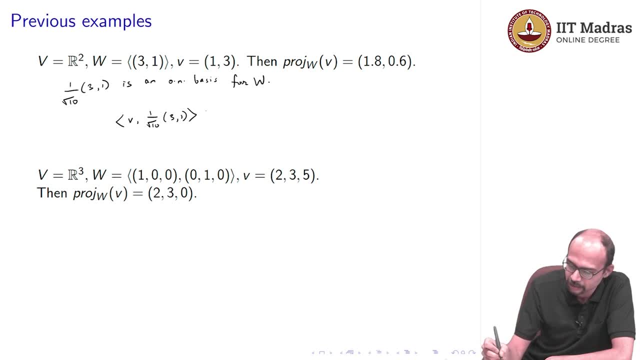 1 by root 10, 3 comma 1 and multiply it by the basis vector. This, whatever value you get, you multiply it to the basis vector. So this is 3 comma 1 and this is the projection. So let us compute what that is. So if you take this in a product, you get: 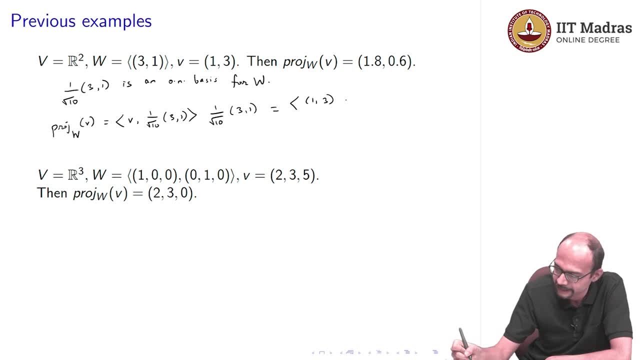 so this is in a product of 1 comma 3, I can take that 1 by root 10 out and I have 1 by root 10 again here. So I get 1 by 10, 3 comma 1 and this in a product is 1 times 3 plus 3 times 1. 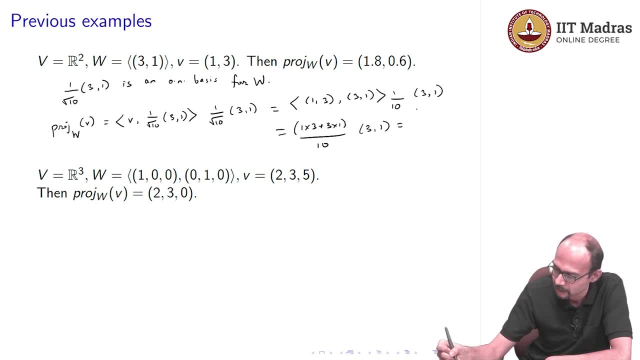 by 10, 3 comma 1.. So this is 6 by 10, 3 comma 1.. And now, if you multiply, you get 1.8 comma 0.6.. So this is exactly what we had over here. 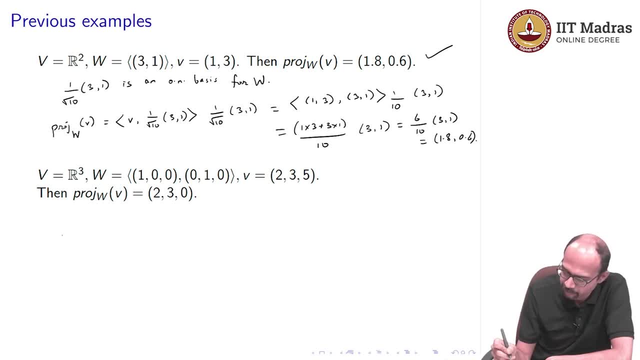 Similarly here. well, in this case, the, you have an orthonormal basis given, So this is the standard vectors, standard basis vectors, So this is an orthonormal basis. So now, what is the projection? 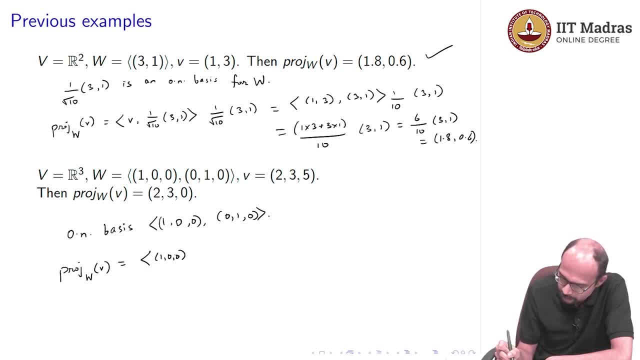 So this is the inner product of 1, 0, 0. or let us write that on the other side, 2, 3, 5 comma 1, 0, 0 multiplied to 1, 0, 0, plus 2, 3, 5 comma 0, 1, 0 multiplied to 0, 1, 0. So if you take this, as in a product, you can multiply this calibrated by 0, 0, 0, multiplied to 1, 0, 0, or through 2,, 3,, 5 comma 0, 0.. So if you calculate what this saying makes this, 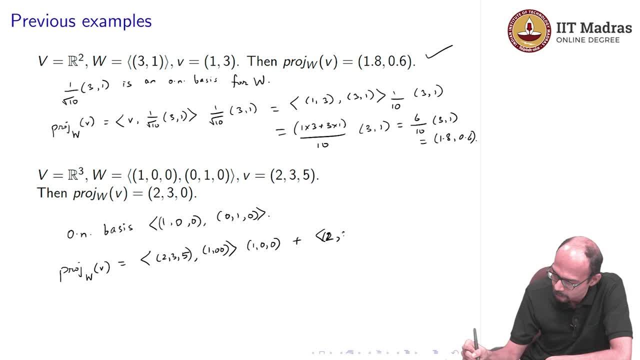 is the product of 0, 0, or let us write that on the other side, just to have an idea. whatever either in terms of faith that let us take that. So this has a specific meaning and certain arrival matrix, or the maximum. 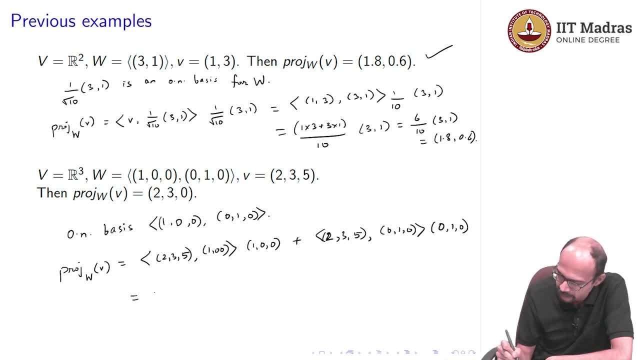 axis emitting these LU eggs, because it is between end and end of theしましたporases. So if you take this in the product, you get 2.. So this is 2 times 1 comma 0 comma 0. And if you take this in the product, you get 3.. So this is 3 comma 0 comma 0. So you 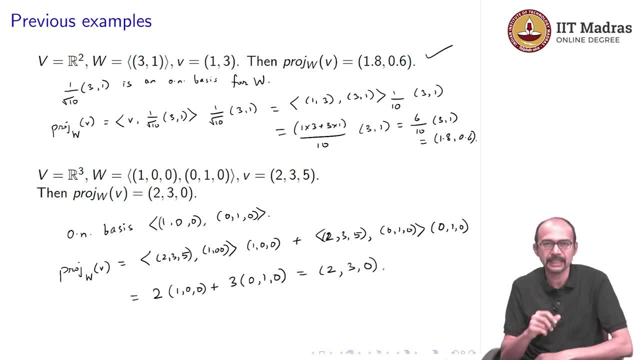 get 2 comma 3 comma 0. So this is exactly what you expect. If you have a vector like this and you take its projection onto the xy plane, that vector will have z coordinate 0, but the x and y coordinate do not change, and that is exactly what you are getting here. 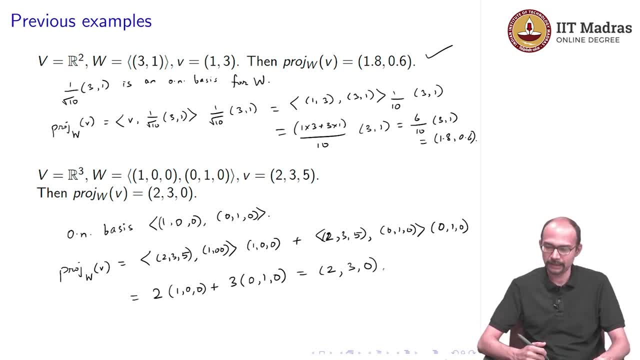 That is exactly the picture that we saw in our second example. So the projection indeed does maintain, does do what we expect it to. I mean, this definition that we have does indeed do what we expect it to do for the usual Euclidean geometry. 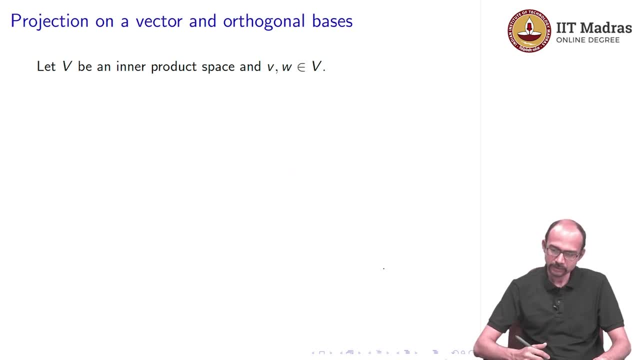 Let us now ask what happens if, instead of an orthonormal basis, you have orthogonal basis. We already saw in that previous example that we had. I think it was 3 comma 1. So we converted it into an orthonormal basis. 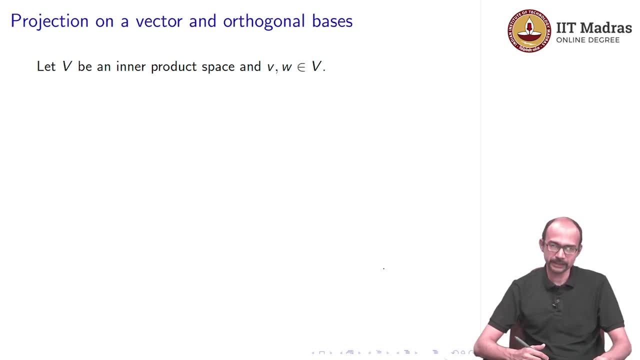 and then we applied the definition, and that is what you can do here as well. So first of all let us define what is projection on a vector. So let V be an inner product space and V and W be vectors in V. 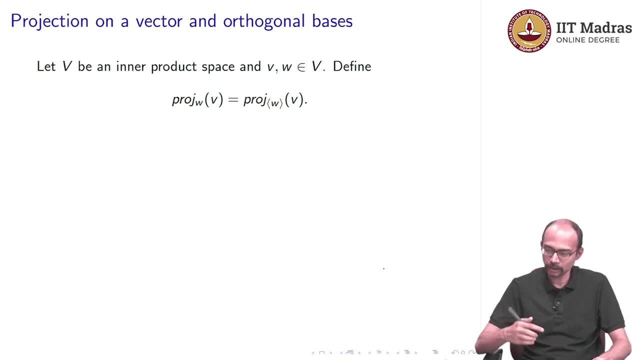 So define the projection of V on W. So now this W, remember, is a vector- is projection of the subspace generated by W. So you take projection of V onto the subspace generated by W. So how do we find this? Well, you take your little w and your little w is a basis. 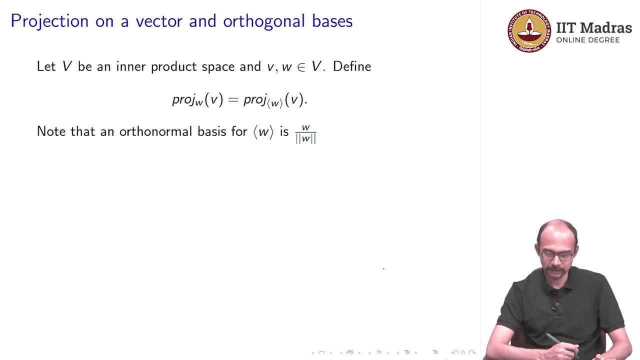 vector for the subspace it generates and you divide it by its norm, So that will give you an orthonormal basis. This is only one basis vector here, So there is no question of orthogonality. So the only thing you have to ensure is that the norm is 1, which you 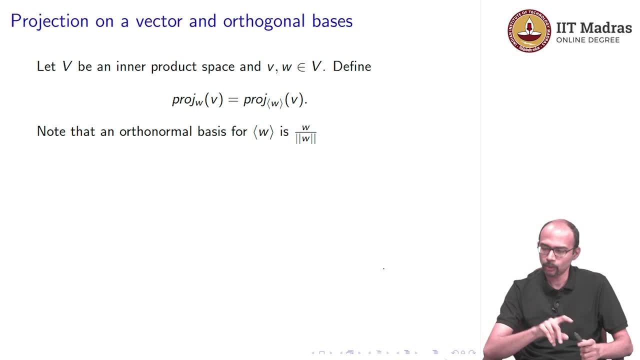 can do by dividing by its norm. Now I should point out that if it so happens that W is 0, then you do not have to do all of this. The projection is just defined to be 0, because there is nothing else you can. 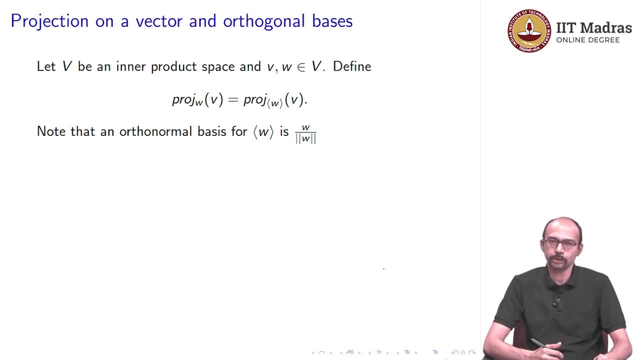 do So. assuming it is non-zero, you can divide by its norm. So once you divide by its norm, you get W by norm of W, which is an orthonormal basis for the subspace generated by W, And now you can take the projection. So the projection of V on W is, by definition, V comma inner. 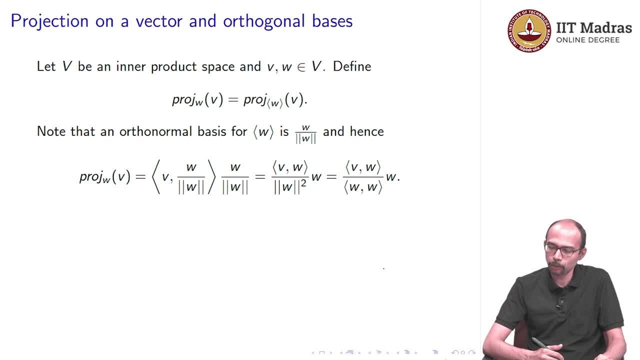 product of V comma W by norm W, times W by norm W, which, if you work out, this is what we did in our previous example as also in the first example with R2.. So you can see, this is the beginning. So here we get the inner product of V comma W. you can take the. 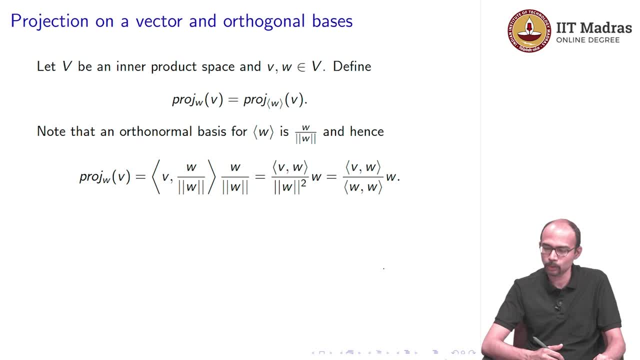 norm out and you get a square of the norm in the denominator from the two norms And then you can write it as inner product of V comma W divided by norm of W comma W times W. So this is the expression we got right at the beginning in the first slide of this. 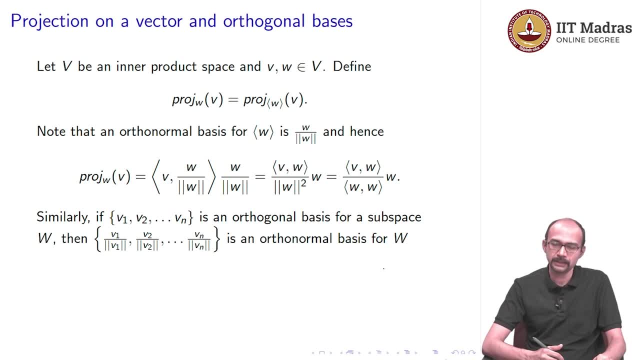 video. So now we can expand this. If you have V1,, V2, Vn as an orthonormal orthogonal basis for a subspace W, Then you can divide each of them by their norms and that will give you an orthonormal. 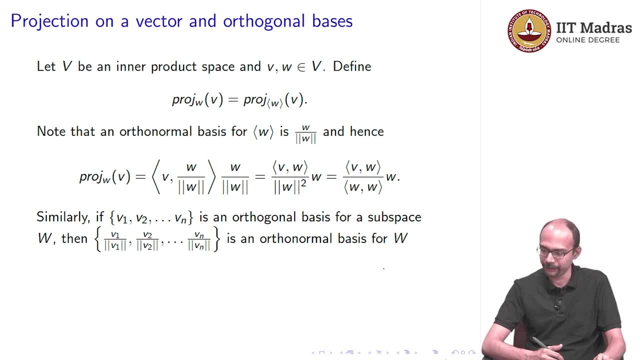 basis. This is what we have seen in the previous video And that is why if you take the projection, that means you are taking the projection with each of those Vi by norm Vi and then the inner product with each Vi comma, norm Vi, multiplying by Vi by norm Vi and taking the sum. And if 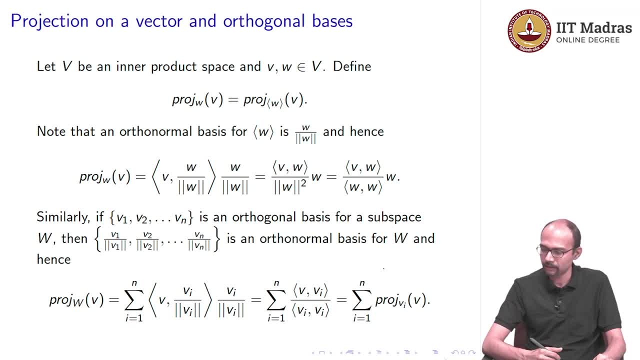 you work it out, that means you get summation: V comma inner product of V comma Vi times inner product. So this is the inner product of Vi comma Vi divided by V inner product of Vi comma Vi. and here there is a typo. This should be times Vi. And then this thing here is exactly what. 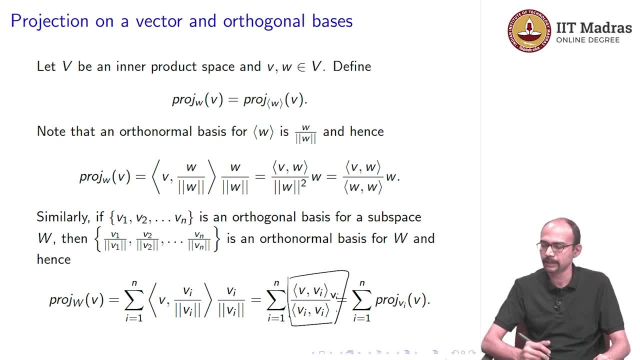 we call the projection of V on Vi. So you can write it as a sum of projection of V on Vi, So the sum. so if you have an orthogonal basis projection of V on W, you can just write it as a sum of the projections on each of the basis vectors. So that is what you. 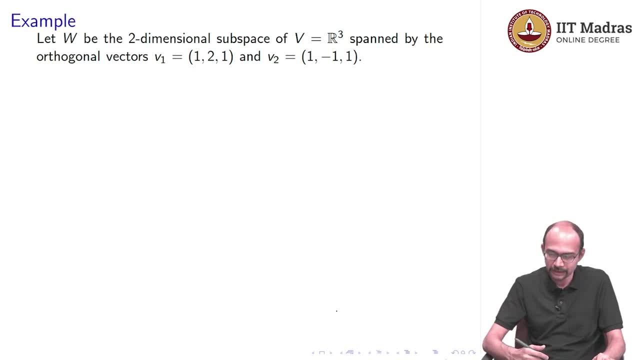 can do So, thank you. So that is my analysis for today. I would like to conclude today's lecture, Thank you. that is the upshot of this argument here. So let us do an example. So let W be. the two-dimensional subspace of V is R3, spanned by the orthogonal vectors. 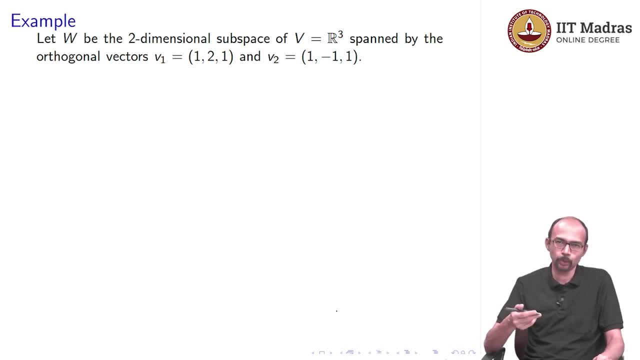 1, 2, 1 and 1 minus 1, 1.. By the way, you do not have to take my word that these are orthogonal. You can take the inner product. I should also again remind you that if no inner product is, 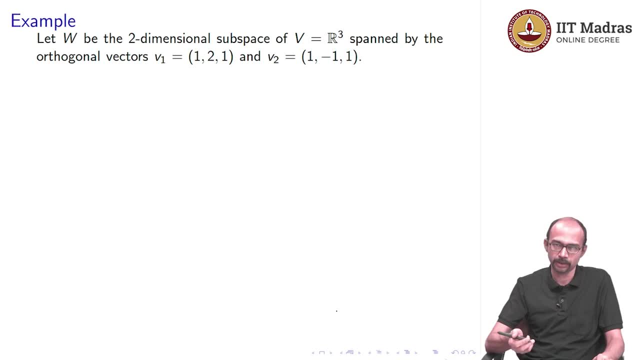 specified, then by default it is the standard inner product for Rn. So here that means it is a dot product. So if you take the dot product you get 1 minus 2 plus 1, which is 0. So these: 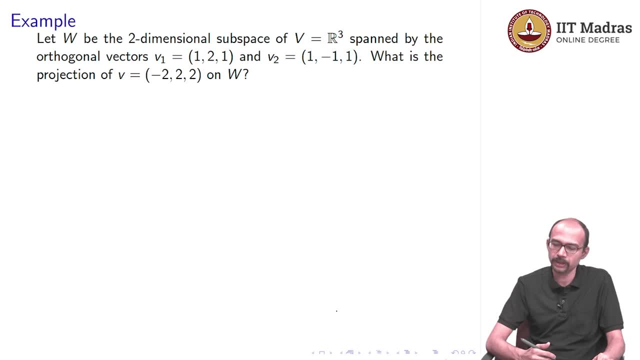 are orthogonal. So what is the projection of V is minus 2, 2,. 2 on W. We find out each of these individual projections. So the projection of V on V1 is, by definition, as we saw, inner product. 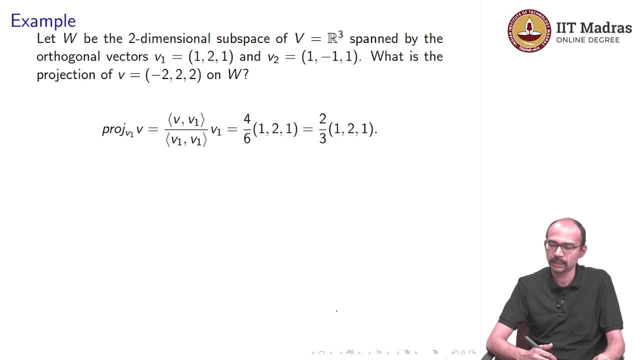 V comma, V1, divided by the inner product V1, V1 times V1, which, if you work out, gives you two thirds: 1, 2, 1.. So the numerator is minus 2 plus 4 plus 2.. So minus 2 plus 4 plus 2 is just 4. 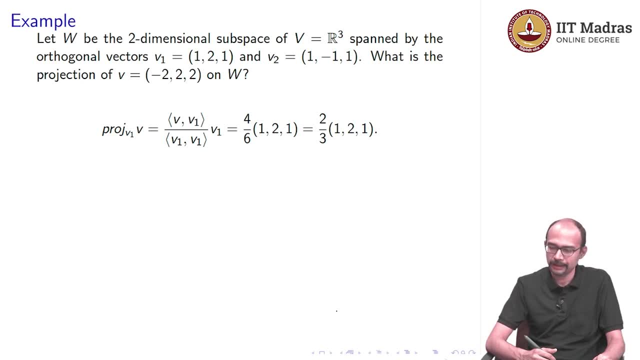 and the denominator is 1 plus 4 plus 1.. So that is 6.. So 4 by 6 times 1 to 1.. So that is what we got. Similarly, if you do it for V2, the numerator is: 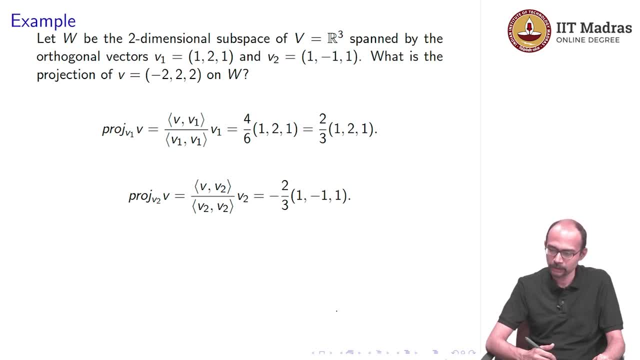 minus 2 minus 2 plus 2.. So that is minus 2, and the denominator is plus 1 plus 1,, so that is 3.. So you get minus two-thirds times 1 minus 1, 1.. And now the 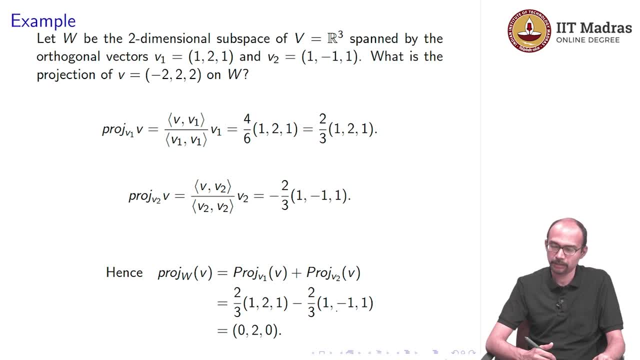 projection of V on W, meaning the subspace is where you add these projections up. So that is given by. so this should not be a capital. this was a small, So that is two-third one to one minus two-third 1 minus 1, 1, which gives you two-third times 2 plus 1 in the. 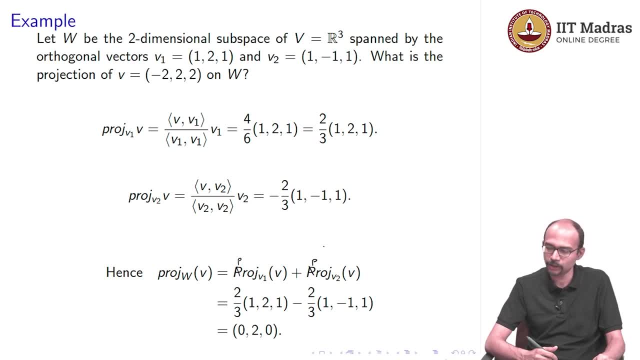 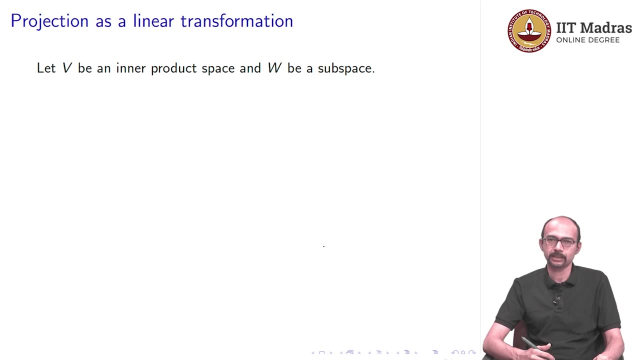 second coordinate and zeros in the other coordinates. So that gives you 0 to 0.. So that is the projection of V on this subspace W. So at the end let us talk about projection as a linear transformation. So we have studied. 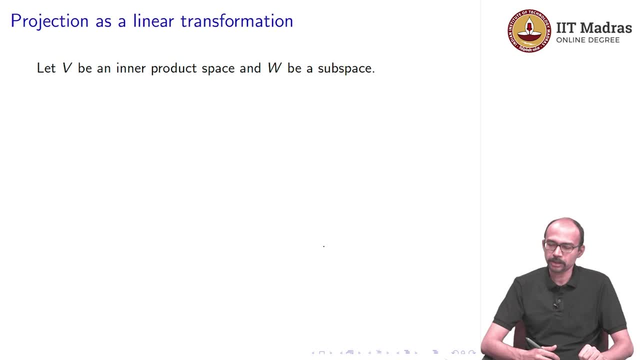 the notion of linear transformation. So we have studied the notion of linear transformation, notion of a linear transformation. So let V be an inner product space and W be a subspace, Then the projection of vectors in V to W is a linear transformation from V to V with image. 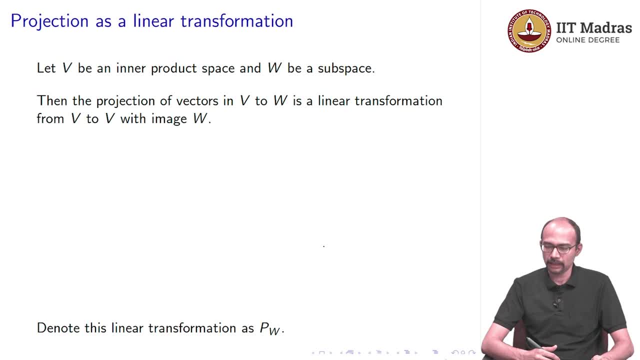 W. So what do we mean by this? Let us study that in a second. Before that, let us remark that we denote this linear transformation as Pw. What is Pw? Let us see what is Pw. So Pw of V, we are saying, is defined as projection of V on W. This is Pw of V, And what do we? 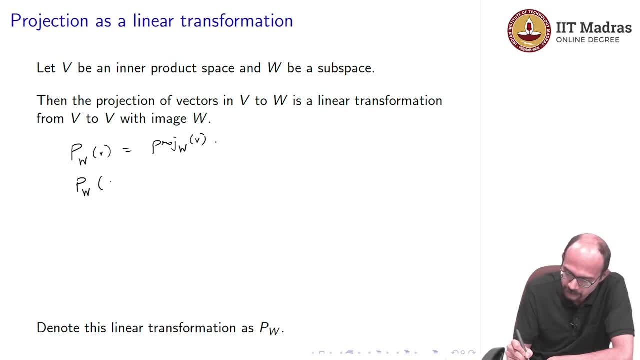 need for a linear transformation to work. for this to be a linear transformation, We need that if you take two vectors, V1 and V2, this is Pw of V1 plus Pw of V2.. And we need: if you take Pw of V2, you will get Pw of V1 plus Pw of V2.. 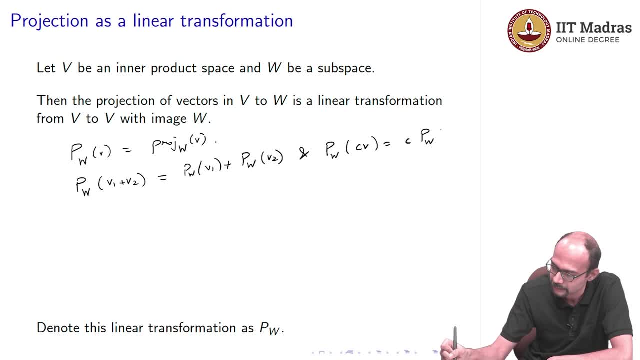 So some constant times V, you get C times Pw of V. This is, if we know these two, then this is a definition of Pw being a linear transformation. So, given a V, we get a new vector in V which is a projection vector, And actually this vector is in W, So it has. 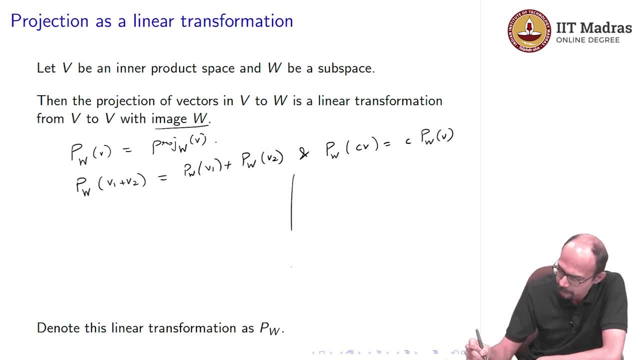 image W. That is what this is saying. So let us maybe quickly run through these proofs. So the idea here is the following: We choose an orthonormal basis, So choose orthonormal basis. let us say W1 through Wn. 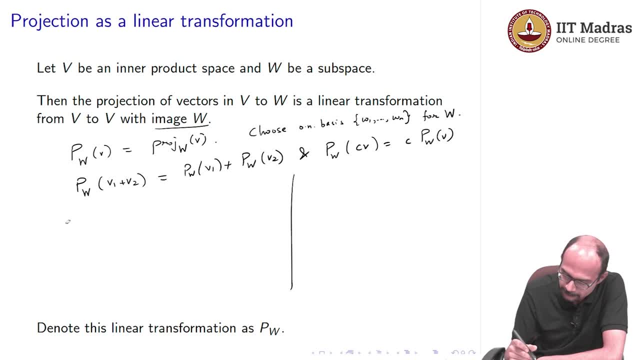 for W, Then, by definition, this thing on the left is summation. we just saw this. This is summation of: well, first of all, by definition, this is projection of V1 through Wn. So we use the V1 plus V2 on W, which we just saw was the projection, the sum of the projections. 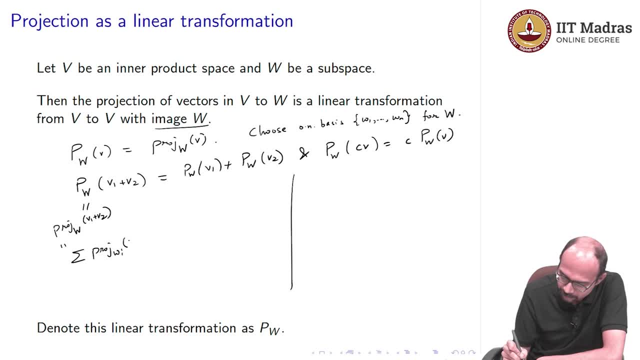 on each Wi. But what is this? By definition, this is the inner product of V1 plus V2, Wi times Wi And then sum 1 through n. But then we can make this into two different terms: v1 comma wi times wi plus v2 comma. 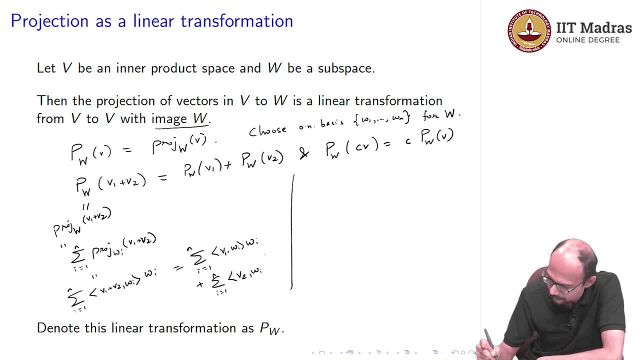 wi, which is v1 comma. wi, so times wi, And this is exactly this term. this is exactly this term. So that is why the projection of v1 plus v2 is a projection of v1 plus projection of v2.. And how about the other part? 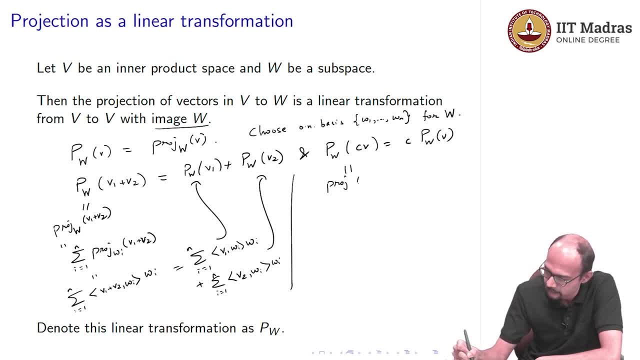 So pw of cv, by definition is projection of cv on w, which, again by definition is summation, is 1 through n. So I will directly write this at this point: This is cv comma wi. So cv comma wi times wi. you can take the c out and then you can remove it all the way. 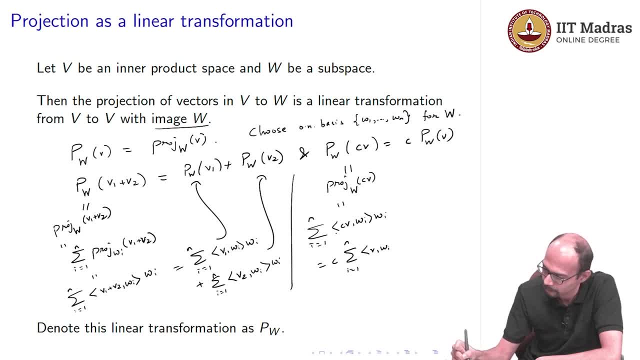 out of the sum as well, the c times summation: v comma, wi times wi, but which is exactly this, So that that is the proof that it is indeed a linear transformation. So what are we saying really? I mean, if you think carefully of what we are saying, it is the following: 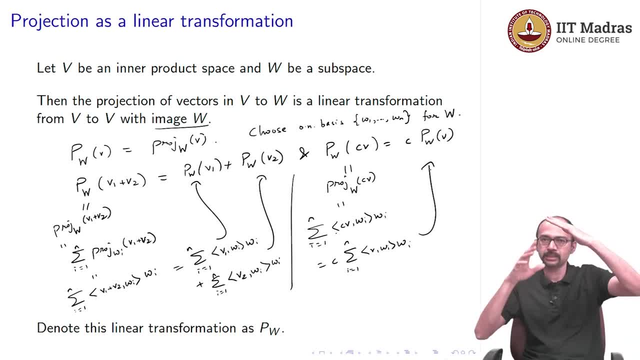 The projection is some kind of taking shadows. So this is saying: if the length of your vector is larger, then the shadow is equal. It is equivalently larger. This makes perfect sense. That is what this second part is saying. And the other part is saying if you take the sums of two vectors, then the resultant vector 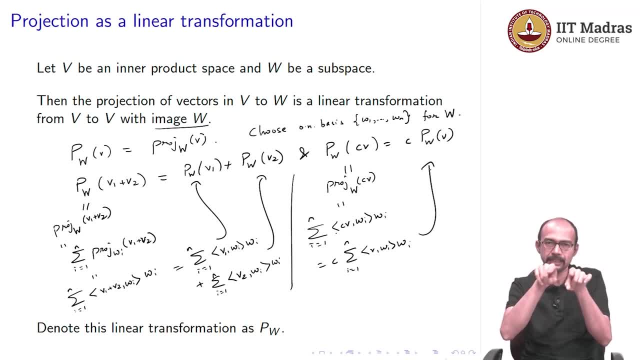 you take its shadow. Instead, if you take the shadows first and then take the sum, you will get the shadow of the resultant. This again, if you think a little about the parallelogram law, this makes perfect sense. So anyway, I have proved it. 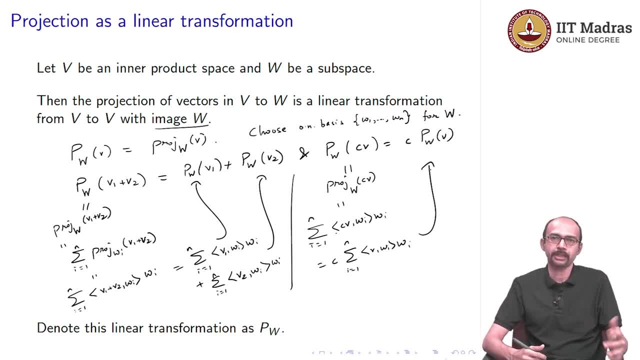 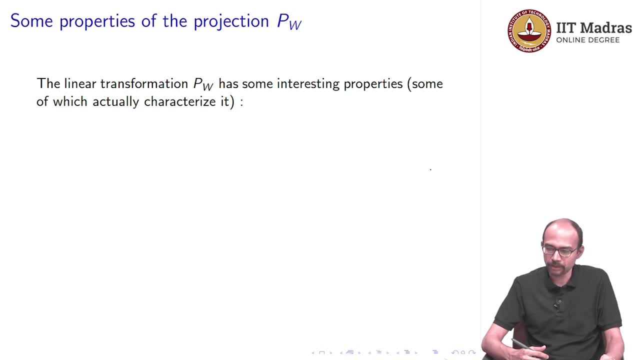 But this is not, I mean even geometrically. this is very natural. Let us quickly look at a few properties of this projection pw. So this is a linear transformation And some of these properties actually characterize it, but I will not expand on what that means. 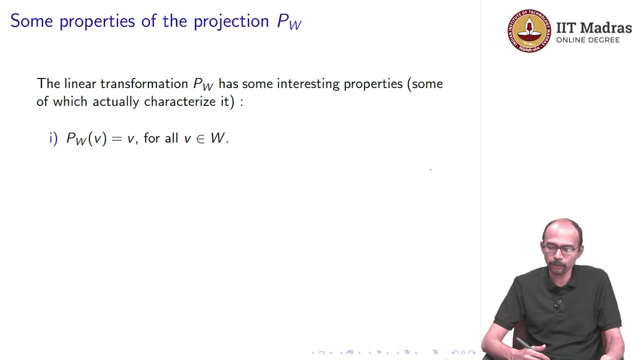 So, first of all, if your v belongs to w, then pw of v is v. Why is that? That is exactly the formula we saw in the previous video. I will come back to this point. Okay, At the end of this slide, range of pw is w. 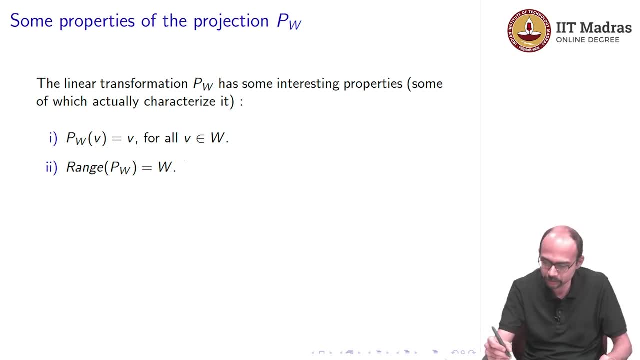 That is what we said. The image of pw is w. Maybe I should. this is range. maybe was not the word we used. We used the word image. That follows from the first point. So let us define this set called w perp. 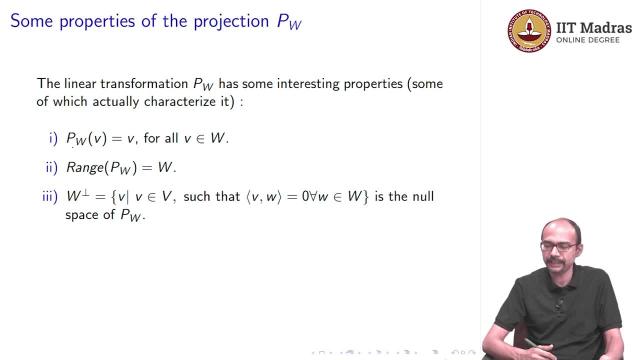 So it is a set of those vectors such that when you take the inner product of such a vector with any element of any vector in w, You get 0. So for example, if, if you have the usual inner product and on R2, and you take the 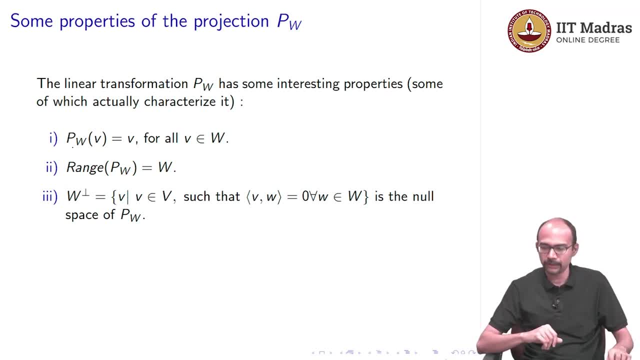 x-axis, then the perp is the y-axis Then. so this is to. we can define this for any inner product space. So w, perp is the set such so defined, And it turns out that this is the null space of pw. 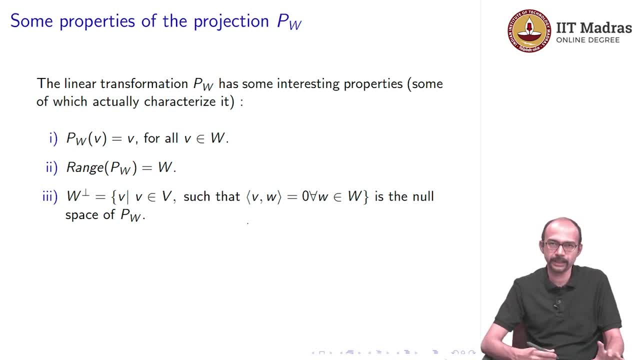 And it. if you look at this definition carefully, It will take your motivation. All right, Thank you very much. minute to prove that Pw squared is Pw. What does this mean? I will come back to this at the end of the slide. 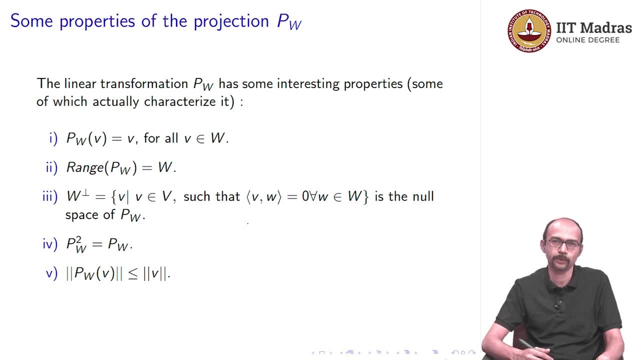 And finally, norm of Pw of v is less than or equal to the norm of v. Very intuitive, because if you take something like this and you are taking its shadow, you are saying that the shadow has smaller length. And now you have to understand here that the length 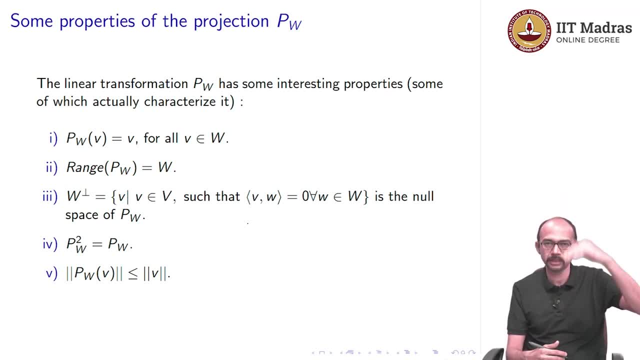 is, if you take a projection in the usual sense, in the perpendicular sense, then this is clear. But if you take your light source elsewhere, then you remember that your norm is also different. So that is why, even if you take it here, you could have a very long shadow, but you are. 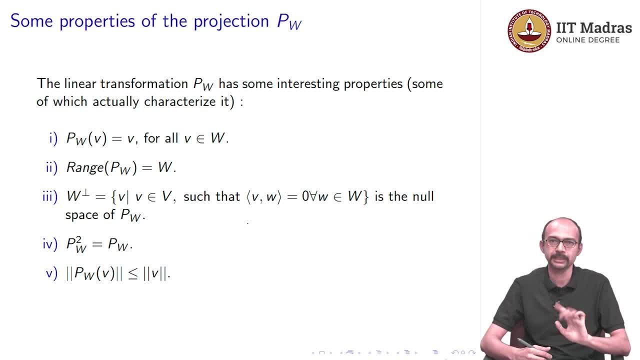 computing length in a different way, So this will still be satisfied. This is a slightly tricky part. I will not expand on this because we probably do not need it in this in this course, But those of you who feel like this is interesting should think of it. 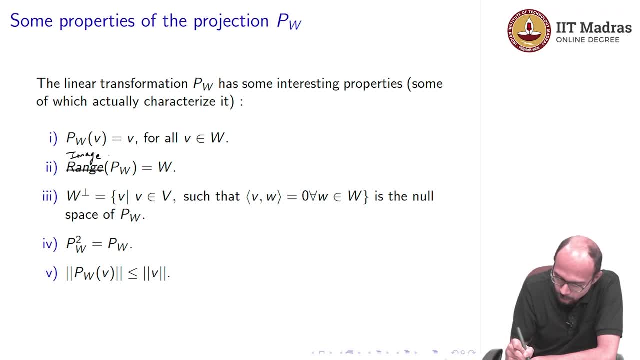 Let me come back to this part about the image. So, first of all, this is called the image. Why is Pw of v equal to v? Well, what is the definition? Choose an orthonormal basis. So this is an orthonormal basis. And then look at v comma, wi times, wi sum over i. Now if 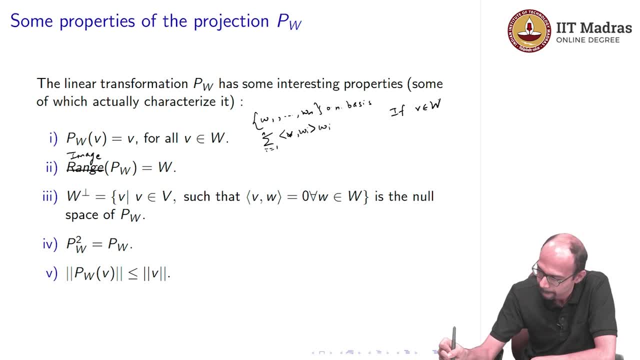 v is in w. so if v is in w, then v summation, ci, wi, because wi is form, a basis. but then what is the ci? We saw in the previous video that the ci? s are exactly these inner products, So the ci. 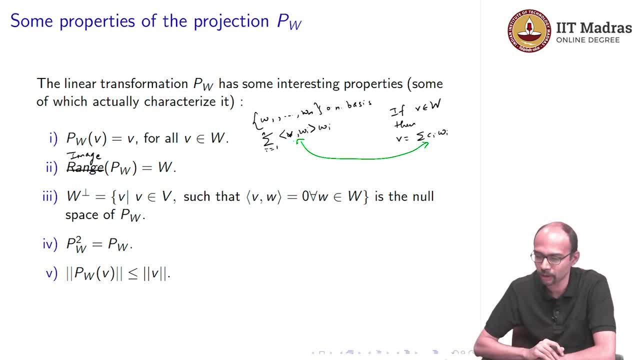 is exactly the inner product v comma wi. So this is so. this is equal to v. That means v is equal to the projection of w. That is the inner product v comma wi. So this is v is equal to v. v comma wi. So this is v comma wi. This is the inner product v comma.